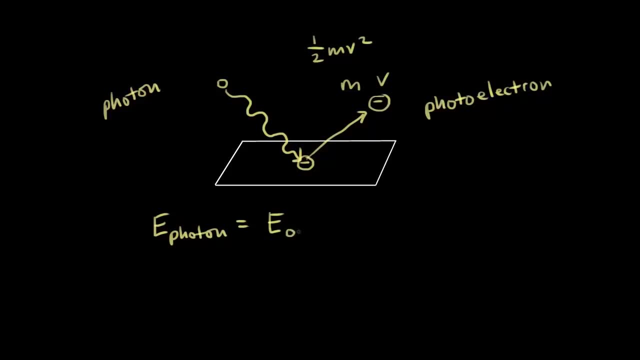 And then the rest of that energy must have gone into the kinetic energy of the electron, And so we can write here: kinetic energy of the photoelectron that was produced, So kinetic energy of the photoelectron. So let's say you wanted to solve for the kinetic energy of that photoelectron. 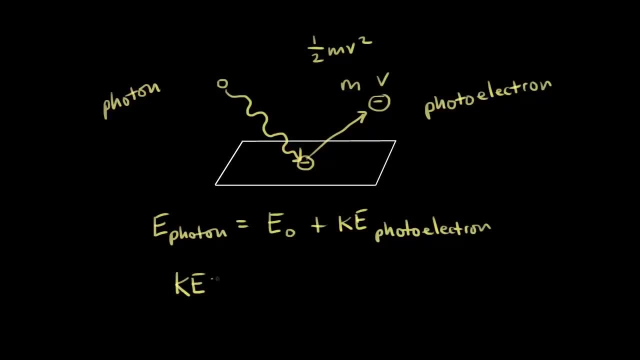 So that would be very simple, Just be: kinetic energy would be equal to the energy of the photon, Energy of the photon Minus the energy that was necessary to free the electron from the metallic surface. And this E naught here, I'm calling it E naught. 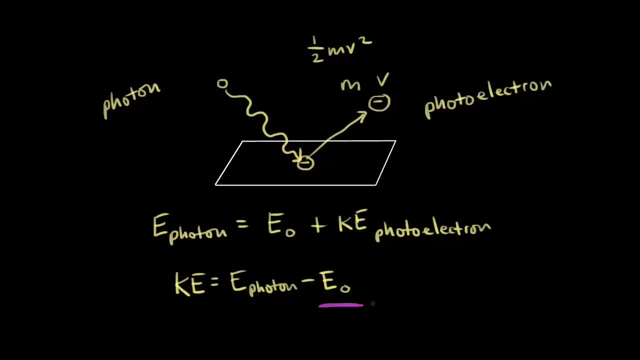 You might see it written differently, A different symbol, But this is the work function. So let me go ahead and write work function here. And the work function is different for every kind of metal. So it's the minimum amount of energy that's necessary to free the electron. 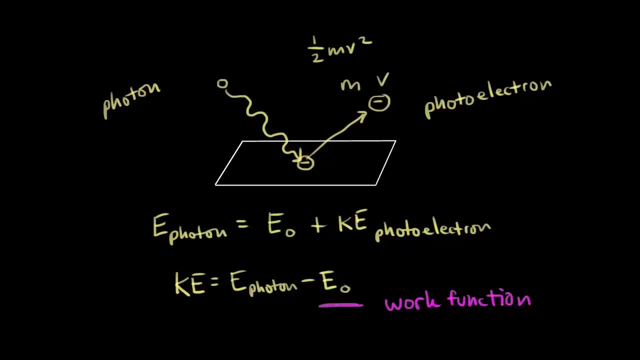 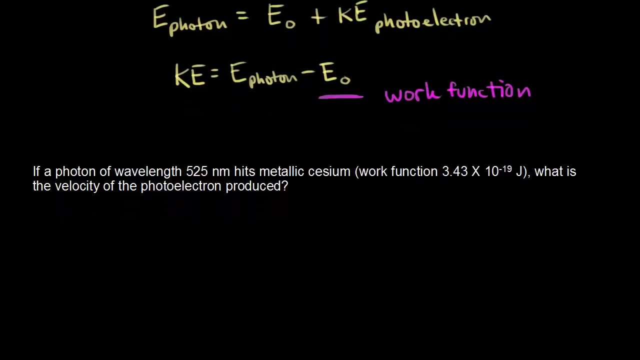 And so obviously that's going to be different depending on what metal you're using. So that's what you're talking about. Alright, let's do a problem. Now that we understand the general idea of the photoelectric effect, Let's look at what this problem asks us. 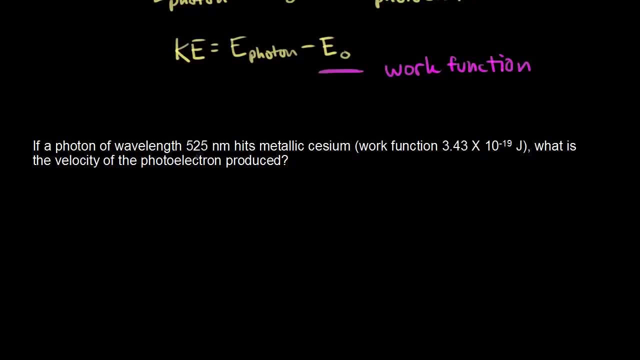 So the problem says: if a photon of wavelength 525 nanometers hits metallic cesium- And so here's the work function for metallic cesium, What is the velocity of the photoelectron produced. So they want to know the velocity of the photoelectron produced. 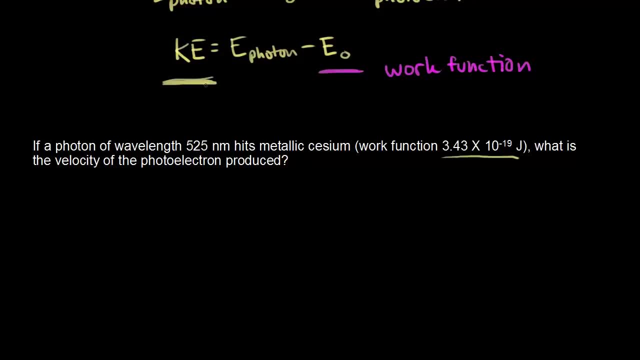 Which we know is hiding in the kinetic energy right here, And we also know what the work function is. So we know what E naught is here. What we don't know is the energy of the photon. So that's what we need to calculate first. 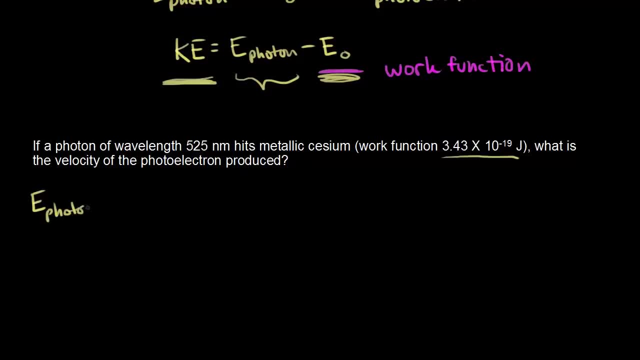 And so the energy of the photon is equal to H, which is Planck's constant times, the frequency which is usually symbolized by nu. So we have the frequency, but they gave us the wavelength in the problem here. They gave us wavelength. 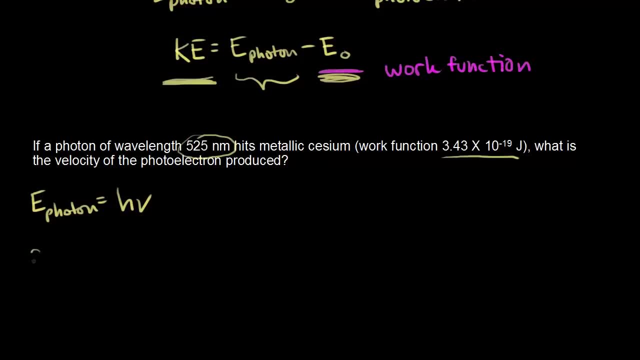 So we need to relate frequency to wavelength And that's related by C, Which is the speed of light, is equal to lambda times nu. So C is the speed of light and that's equal to the frequency times the wavelength, So we can substitute in for the frequency. 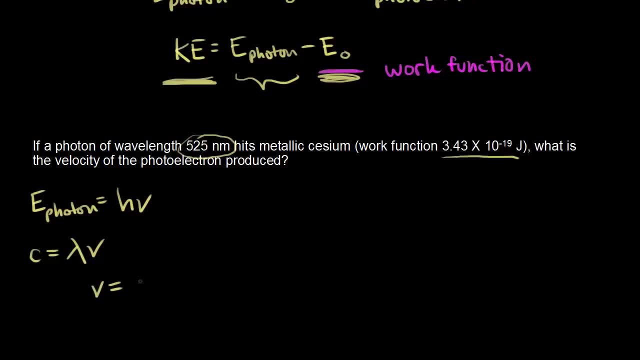 Because we can just use this equation and say that the frequency is equal to the speed of light divided by the wavelength. The frequency is equal to speed of light over lambda, So we can plug that into here And so now we have: the energy of the photon is equal to. 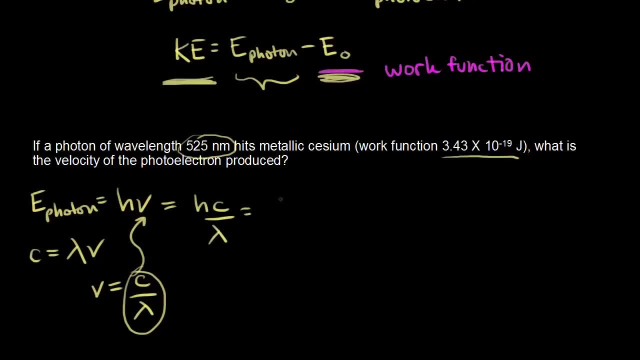 Hc over lambda, And we can plug in those numbers. H is Planck's constant, which is 6.626 times 10 to the negative 34.. So times 10 to the negative 34. here C is the speed of light, which is 2.998 times 10 to the eighth meters over seconds. 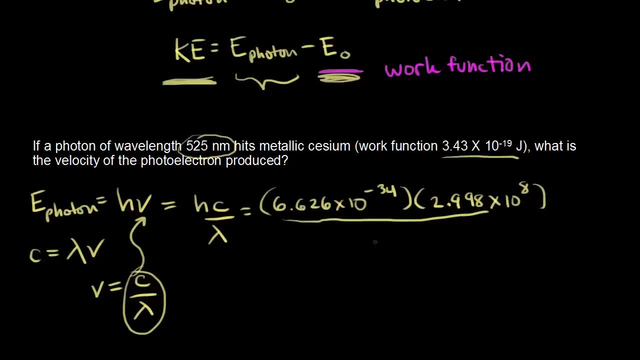 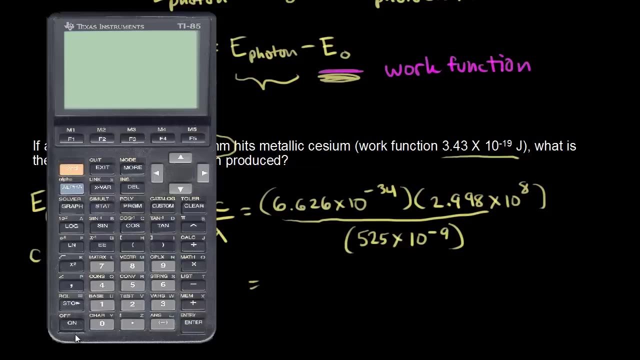 And all over lambda. Lambda is the wavelength, That's 525 nanometers. So 525 times 10 to the negative ninth meters, All right, So let's get out our calculator and calculate the energy of the photon here. So let's go ahead and do that math. 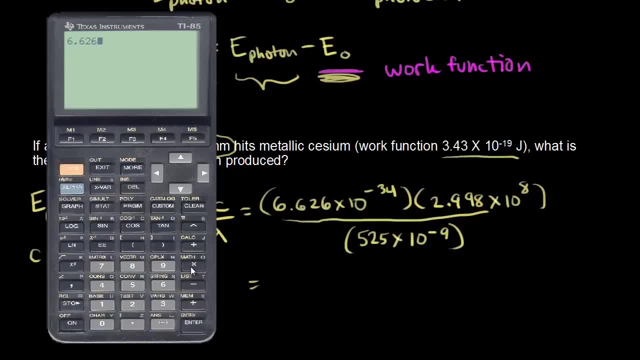 So we have 6.626 times 10 to the negative 34.. And we're going to multiply that number by the speed of light, 2.998 times 10 to the eighth, And we get that number. We're going to divide it by the wavelength. 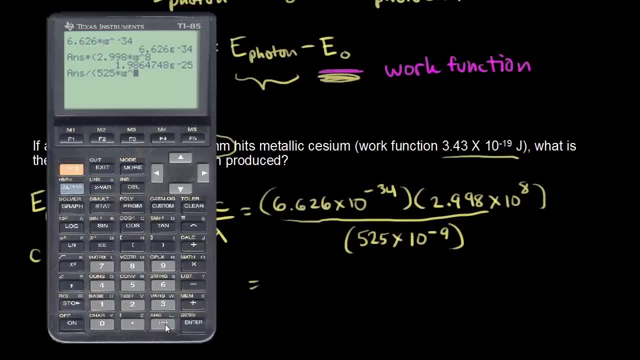 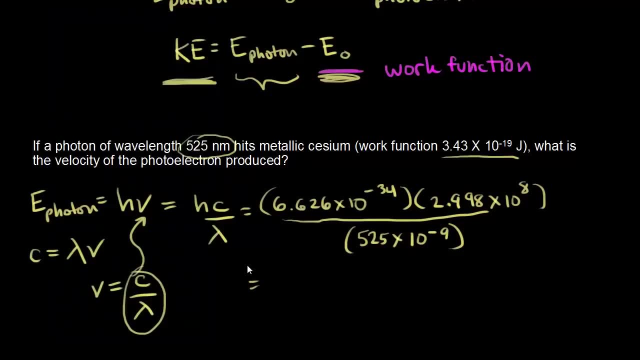 525 times 10 to the negative 9.. And we get 3.78 times 10 to the negative 19.. So let me go ahead and write that down here: 3.78 times 10 to the negative 19.. 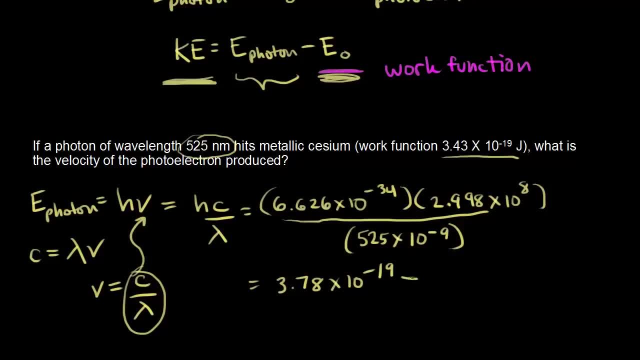 And if you did your units up here you would get joules. And so let's think about this number for a second. 3.78 times 10 to the negative 19 is the energy of the photon, And that energy of the photon is greater. 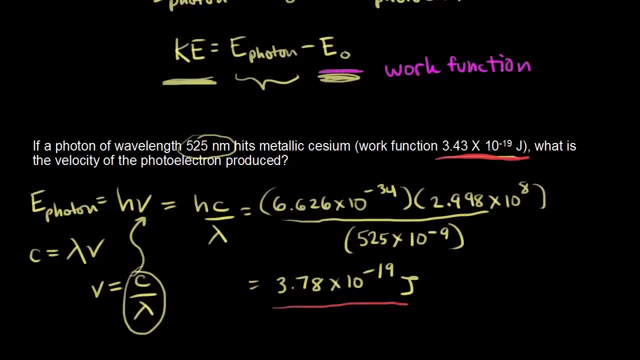 than the work function, Which means that that is a high energy photon. It's able to knock the electron free Because, remember, this number right here is the minimum amount of energy needed to free the electron, And so we've exceeded that minimum amount of energy. 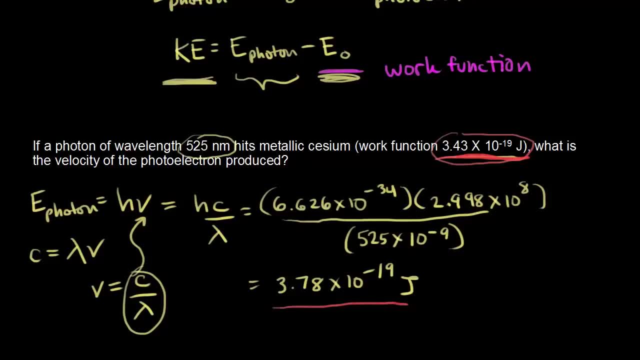 And so we will produce a photoelectron. So this photon is high energy enough to produce a photoelectron. So let's go ahead and find the kinetic energy of the photoelectron that's produced. So we're going to use this equation right up here. 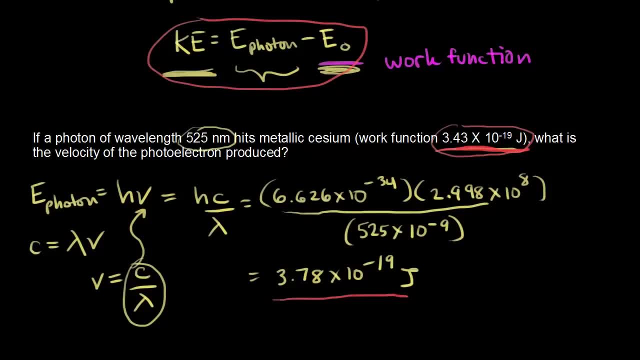 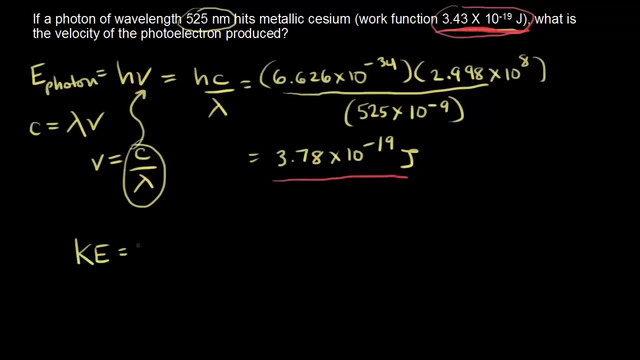 So let me just go and get some more room and I will rewrite that equation. So we have: the kinetic energy of the photoelectron is equal to the energy of the photon minus the work function. So let's plug in our numbers: The energy of the photon was 3.78 times 10 to the negative 19 joules. 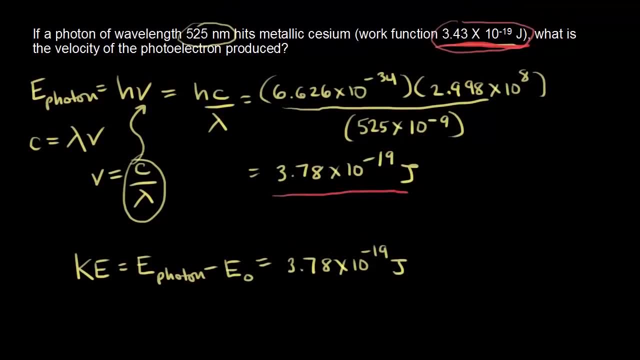 And then the work function is right up. here again It's 3.43.. So minus 3.43 times 10 to the negative 19 joules. So let's get out the calculator again. So from that we're going to subtract the work function. 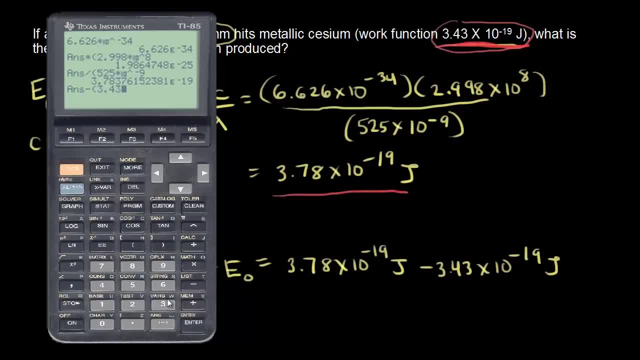 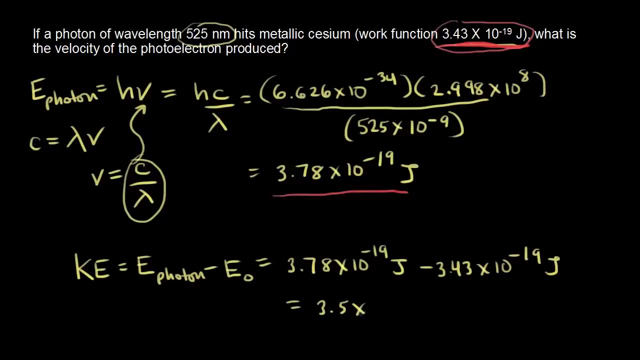 3.43 times 10 to the negative 19.. And we get 3.5 times 10 to the negative 20.. So let's go ahead and write that This is equal to 3.5 times 10 to the negative 20 joules. 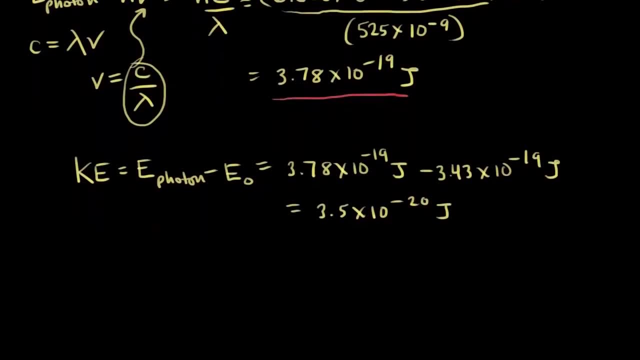 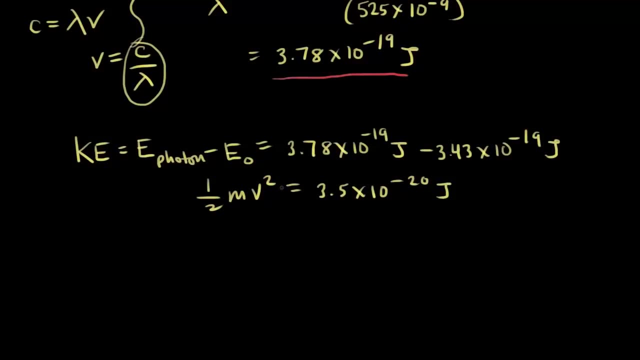 This is equal to the kinetic energy of the photoelectron, And we know that kinetic energy is equal to 1 half mv squared. The problem asked us to solve for the velocity of the photoelectron. So all we have to do is plug in the mass of an electron. 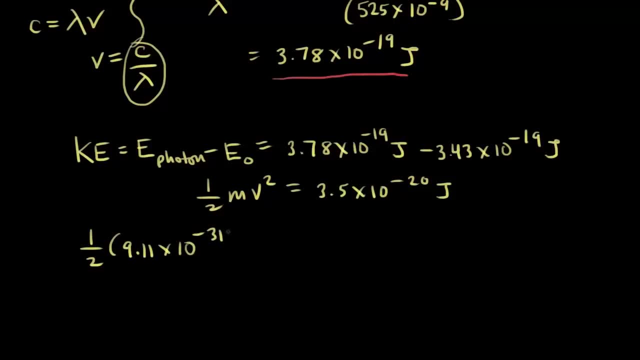 which is 9.11 times 10 to the negative. 31st kilograms times v squared, This is equal to 3.5 times 10 to the negative 20.. So let's do that math. So we take 3.5 times 10 to the negative 20.. 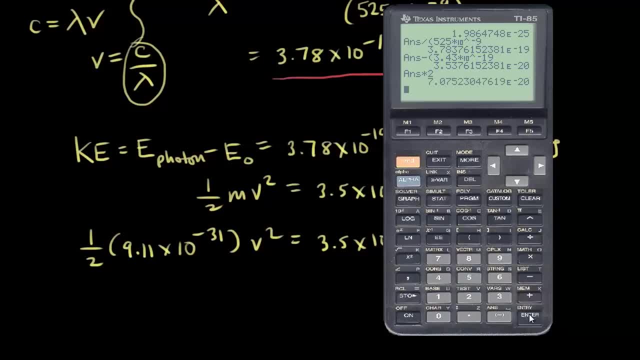 We multiply that by 2. And then we divide by the mass of an electron, 9.11 times 10, to the negative 31st, And this gives us that number which we need to take the square root of, So square root of our answer.